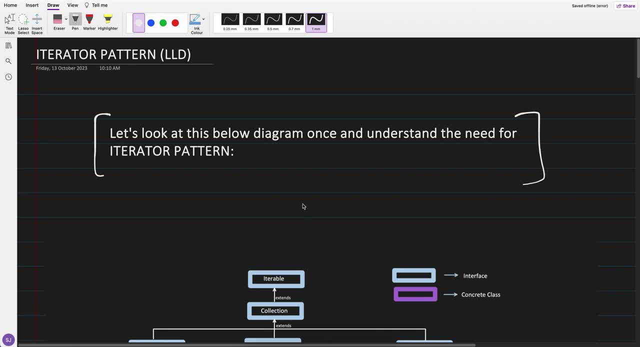 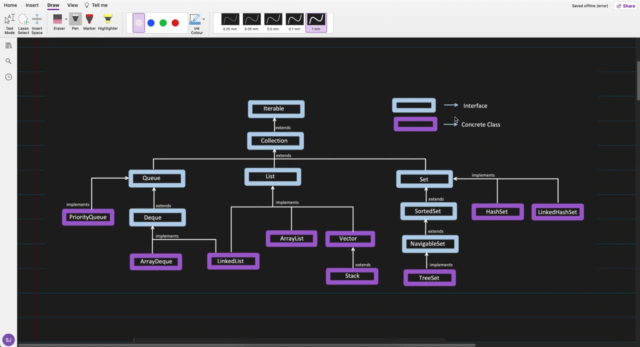 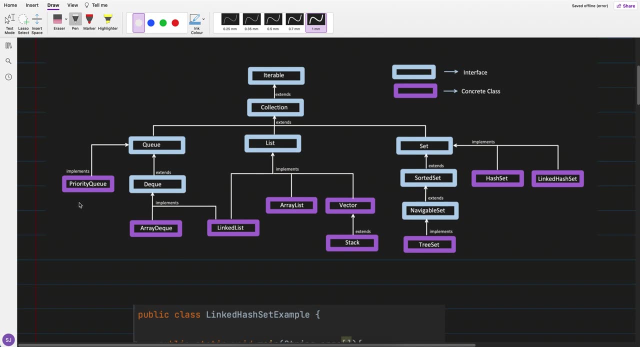 And to understand the usage of iterator pattern, there is no better example than Java collection itself. So this is a diagram which I have taken from a Java playlist right where I have explained the collection in depth. So here if you see that in the Java collections there are different types of collection, like priority queue, array DQ, link list, array list, stack, hash set, linked hash set. 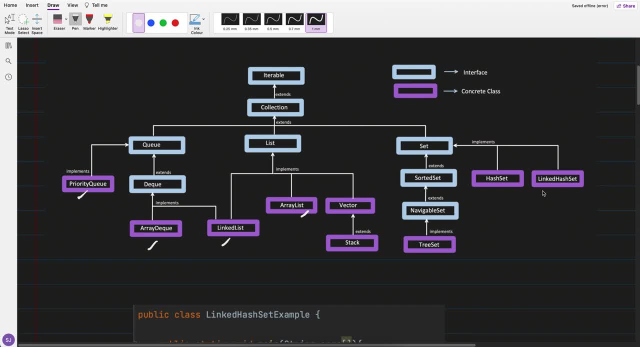 Each stores the data in their particular manner. like link list uses which data structure, Link list, Array list using which data structure Arrays, So each maintains the collect the data in their own manner. But whenever you want to iterate over it, do you client does have to know that? okay, this is linked list I have to access in this particular manner. No, 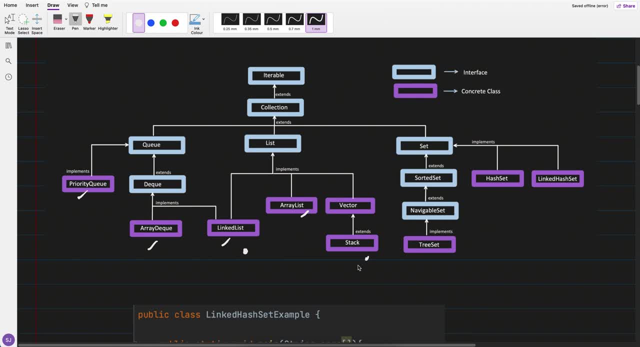 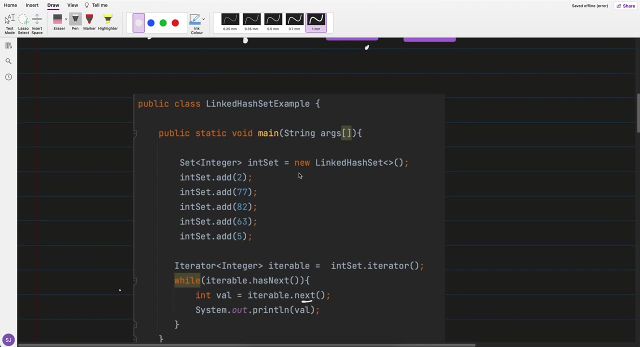 Okay, this is a stack. I need to access the element in this particular manner. Does client bother about the knowledge of how to access the element? No, So for this collection has provided one iterator method, So here in this example, I have created a new linked hash set. 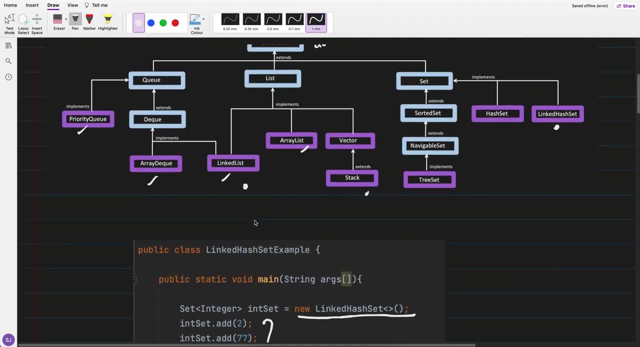 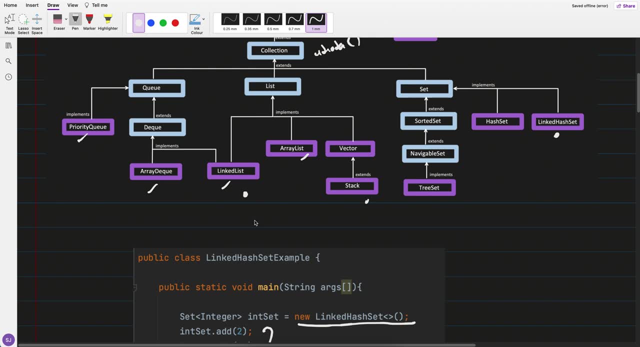 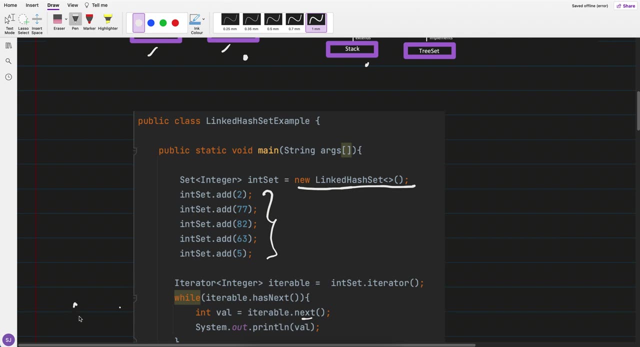 And I have stored certain data. Now it might use the hash map internally right on hash map plus linked list internally to store the data, whatever it would be right, But does client? so this is, let's say, yours, this is your client. 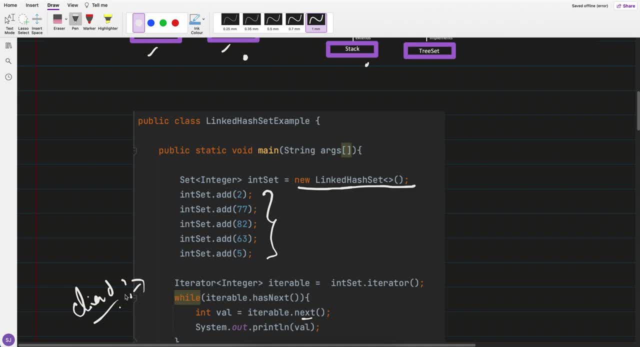 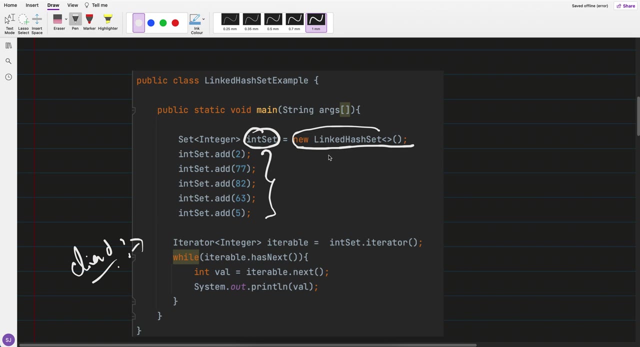 Does client has to have this knowledge about it? like: okay, if I want to iterate, I am accessing linked hash set, So it should be accessed in this manner. No, So client doesn't bother about what type of collection, it is right how the data is stored in this particular collection. 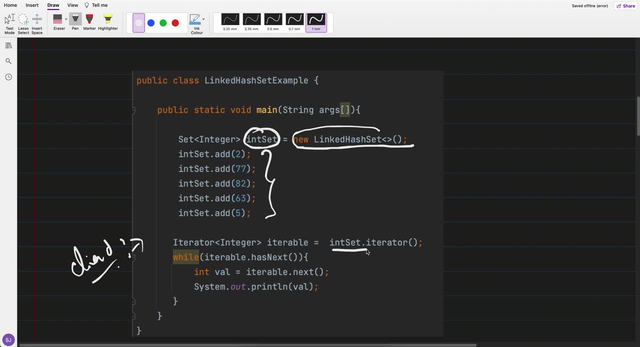 It knows that the collection has given me this iterator method. Once I get this iterator object I can use has next and next, and it will help me to iterate. has next will tell that. okay. is there any more element? If yes, go inside and get me the value. 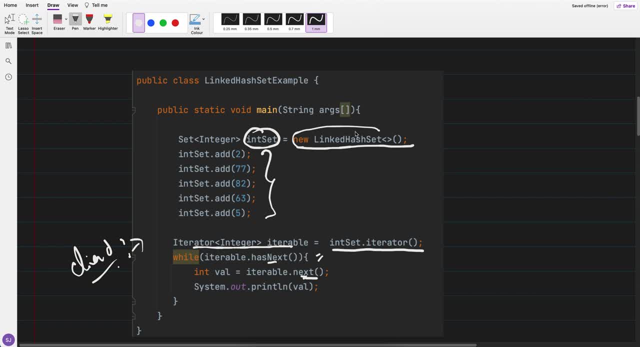 Get me the value out of it, Okay. So now, no matter if I'm using linked hash set here, or priority queue here, or a stack here, This logic will remain the same. This will work for all. Okay, But you can ask me a question right here is how this actually works. 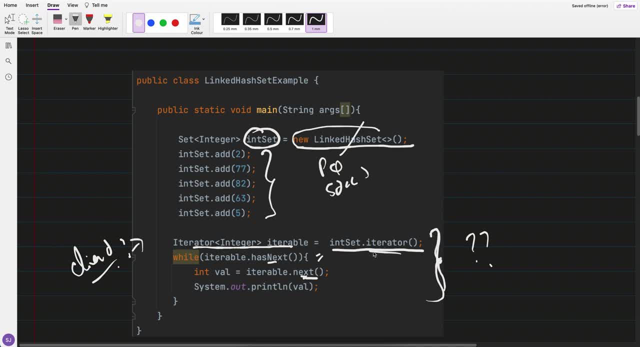 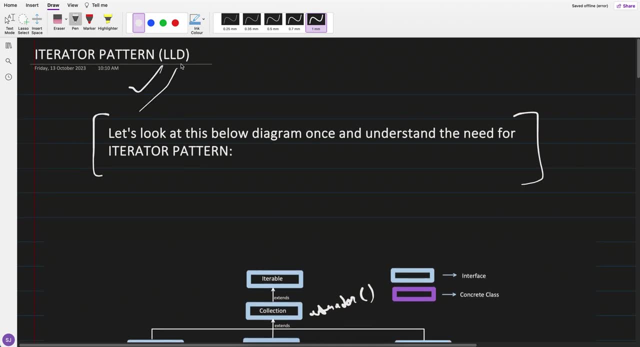 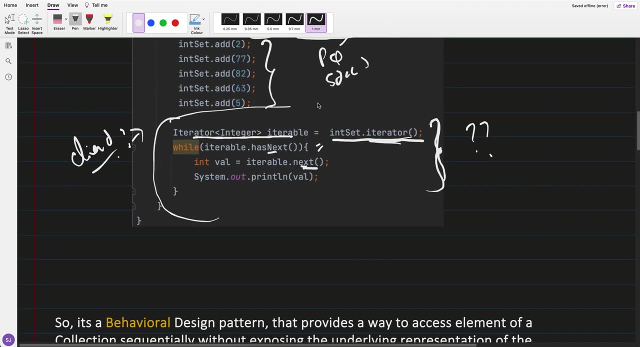 Right How this iterator, which collections expose this iterator method, how this actually works. Actually, that is iterator pattern. So if you understand the iterator pattern, you will get your answer that how this code works for all type of collections. Okay, 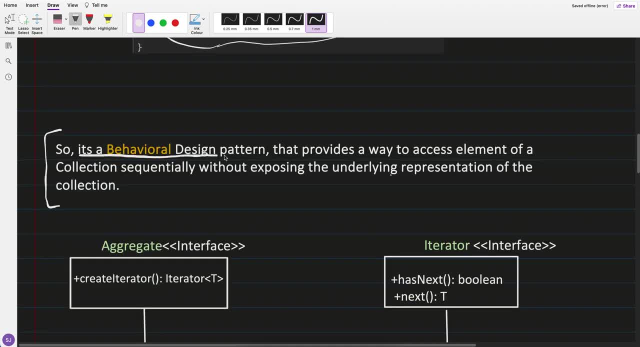 So now let's go into deeper. It is a behavioral design pattern. Okay, That provide a way to access element of a collection sequentially. So that is the first use. It helps you to access element of a collection sequentially Without exposing The underlying representation of the collection. 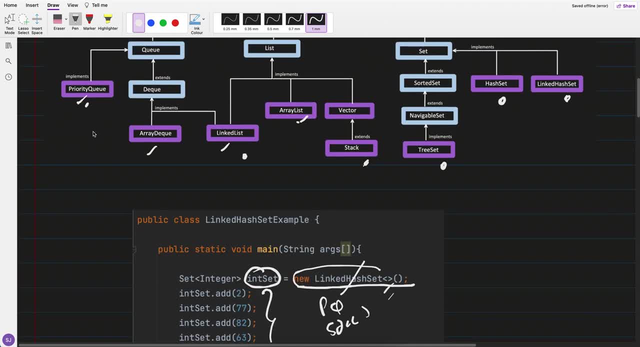 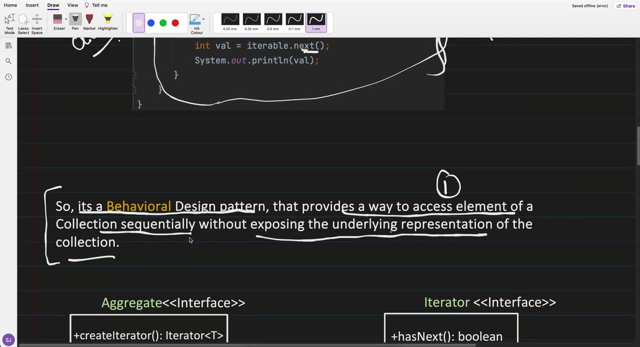 You don't have to worry about what is the underlying data structure used to store the data. You can. it iterator pattern can help you to access the element sequentially. Right, You don't have to worry about the underlying representation of the collection, But how? 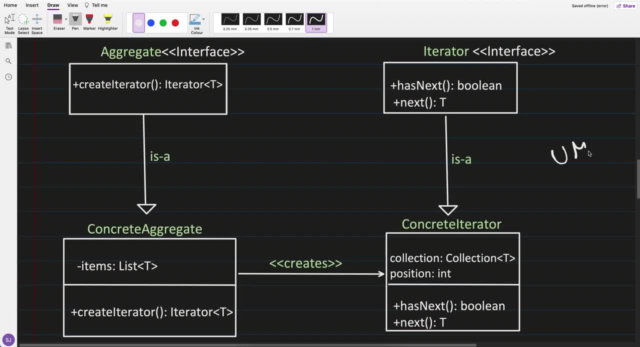 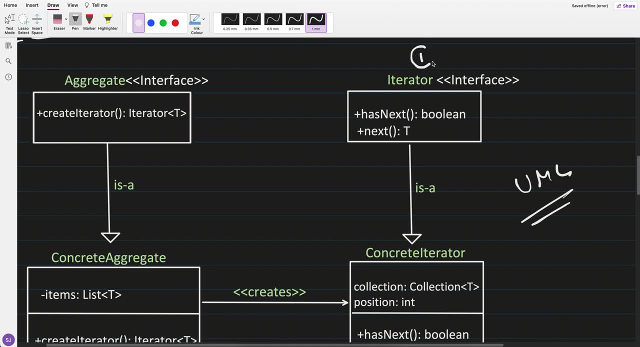 Let's see that. So let's see this UML first, Then we'll see an example. Okay, So here in this UML, What The first we have is iterator Right, This is the first. iterator is the interface which has exposed this to method has next and next: 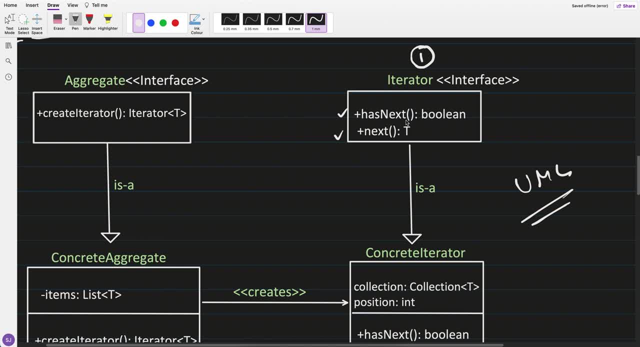 Okay, So has next usage. is that okay? if there are any more element in a collection, it should return true, And when the next method will be involved, it should return the value which the current pointer it's pointing to. Okay, Then it is implemented by. 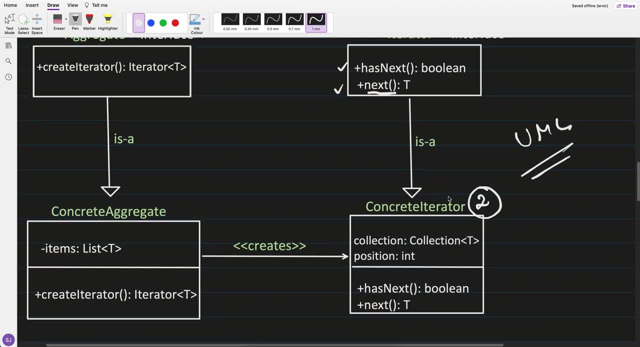 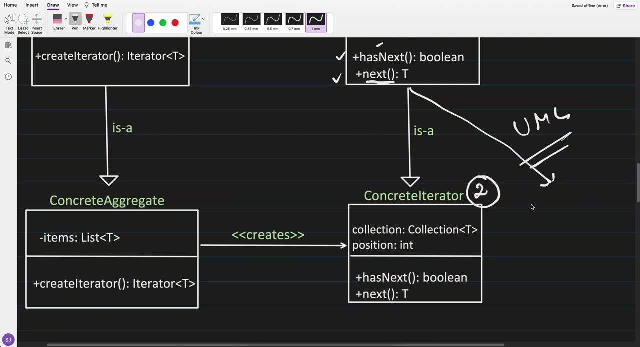 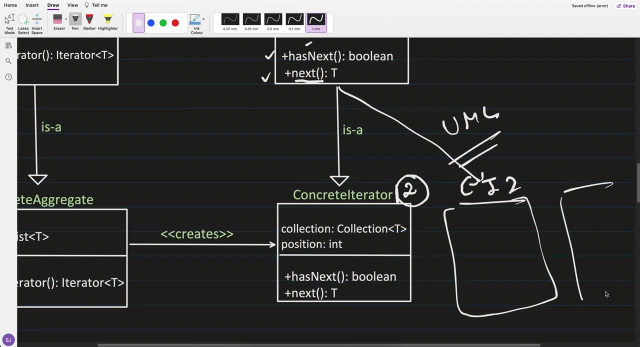 The concrete iterator Right, So the has next and next implementation is done by this. There can be many concrete iterator There can be. So this is concrete iterator one, concrete iterator two. There can be concrete iterator three. There can be many concrete creator and each one can implement their own. has next and next. 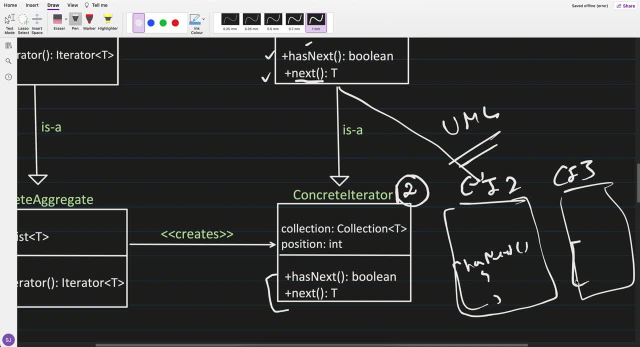 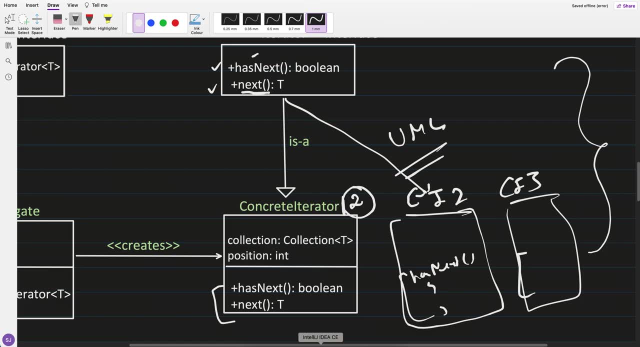 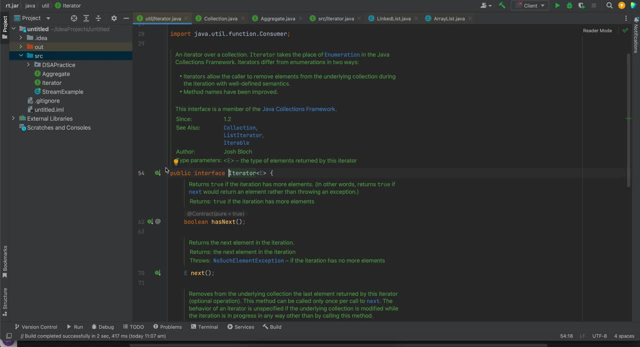 Right, Depending upon the data structure, Data collections. Okay, So now let's first understand this with our Java collections, How it is done. So here, if I go here, inside this collection, So this is the iterator, Iterator, So there is a class called iterator, which is it's an interface. 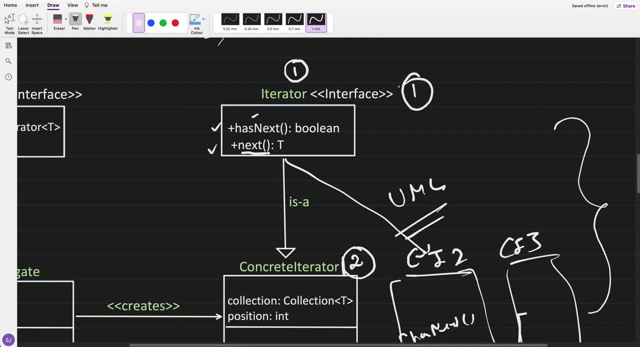 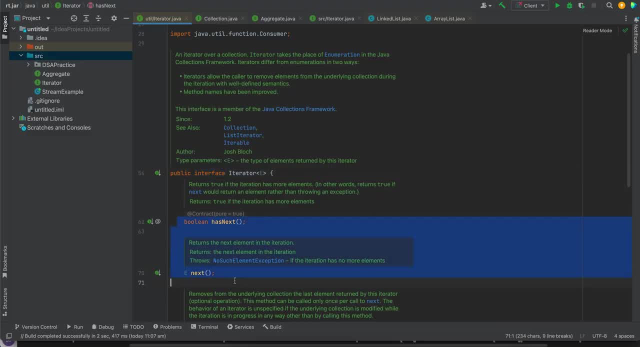 So this is the interface which is first created in Java collections, also package, also iterator Right. It has this two method, has next and next. Now there can be many concrete iterators. Now let's see that which all things have implemented and let's open array list. 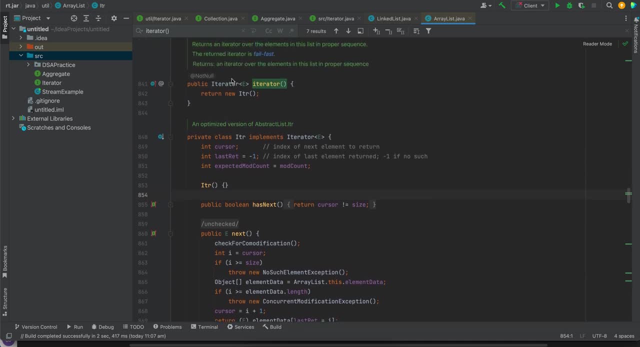 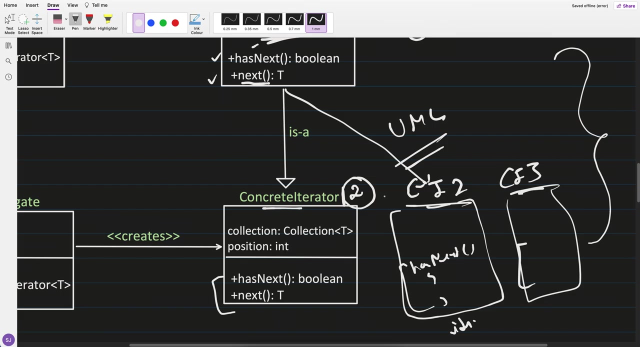 If I open array list Let's see which implements iterator. Okay, So here I TR is the class which is implementing the iterator. So in array list there is something called I TR. Now here, if you see that iterator, Now here, if you see that it has implemented the has. next, if cursor is not equals to the, 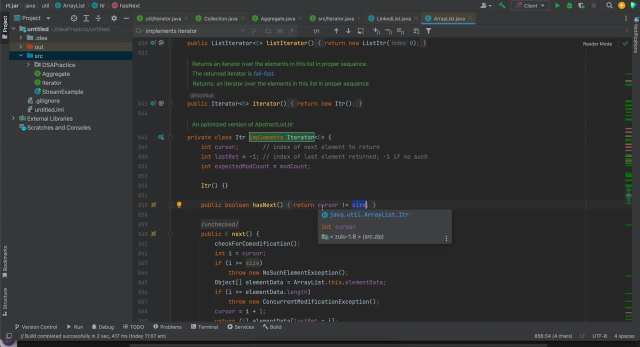 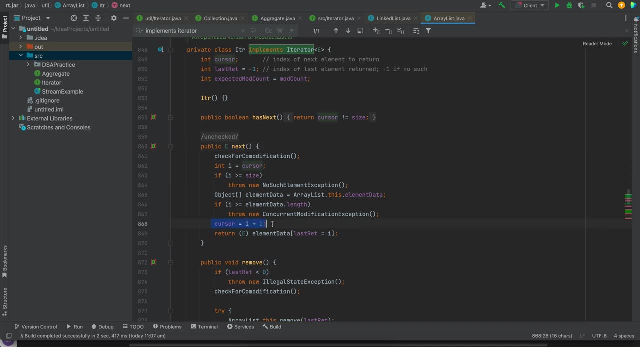 size of the collection means yes, there is still some items and cursor will keep on increasing whenever you call next right, so cursor it will. i plus i plus one right and the next will return the element. okay, so it has its own, because in the array list the collection 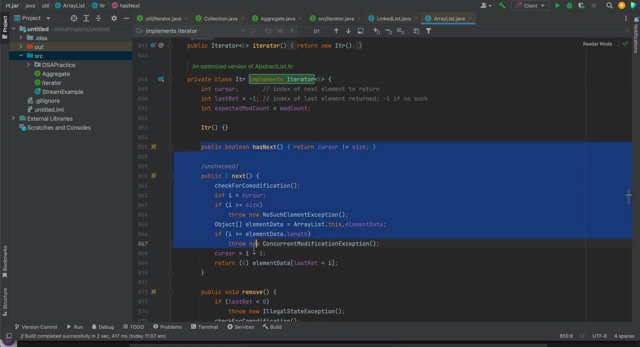 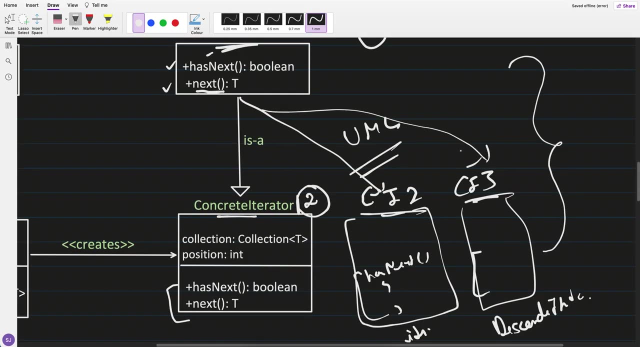 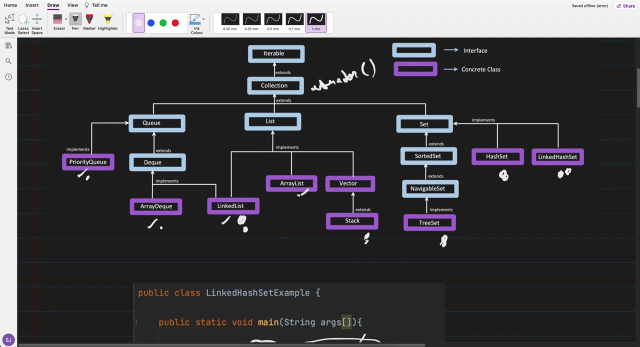 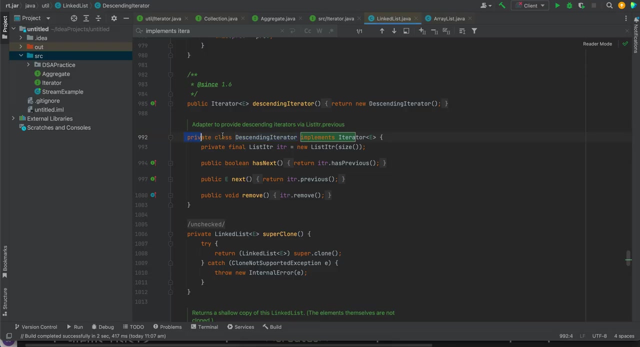 it has to work. so it has written its own logic how to fetch the next element. so what am trying to say? that here you can have as many iterator as possible. so each one, each class here has implemented the iterator. they have created a class. you can say that they. 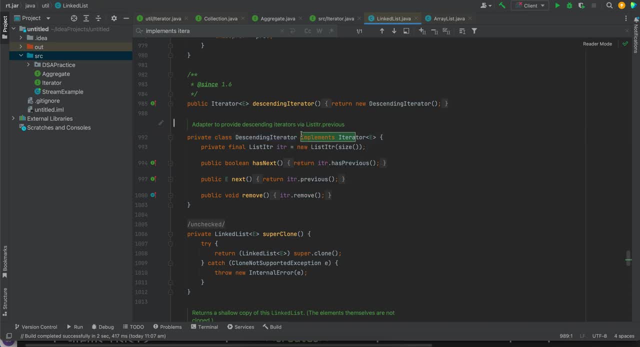 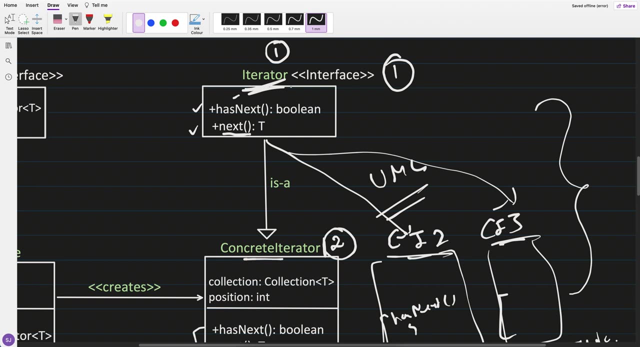 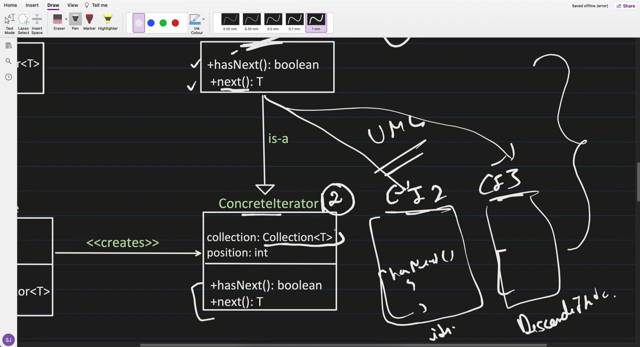 have created a class, local class, where they have implemented the iterator. implement this iterator and implement this- two methods so we can have for this iterator, we can have many right iterators right and they work on this collections. whatever the collection, if it is a linked list, they know that how to do has next and next right. so 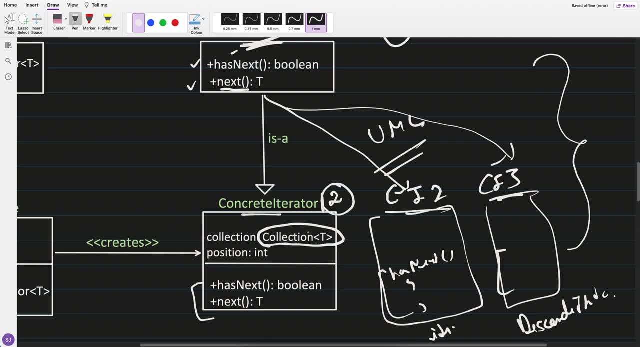 this collection, we will set it up. i will show you an example. so if this collection is, let's say, an array, they know that, ok, how to fetch it. if it is a stack, they know how to fetch, has next and next right. so they work on this collection and perform this so we can have 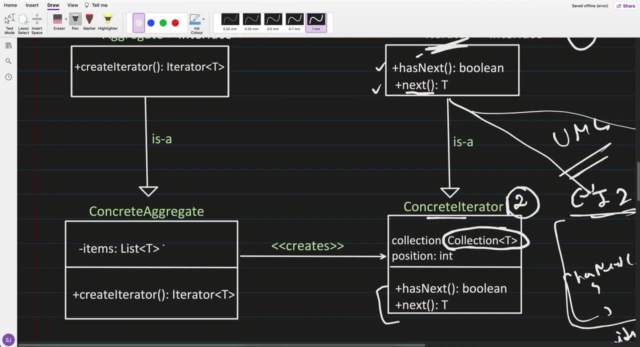 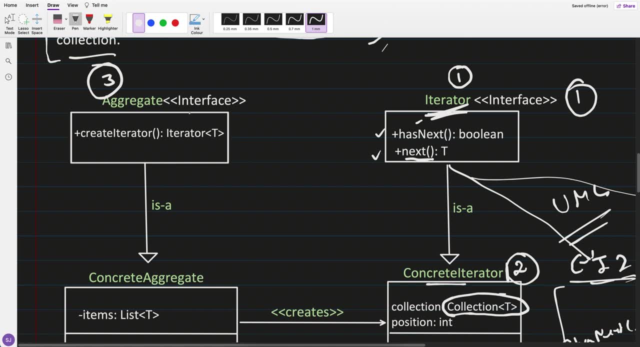 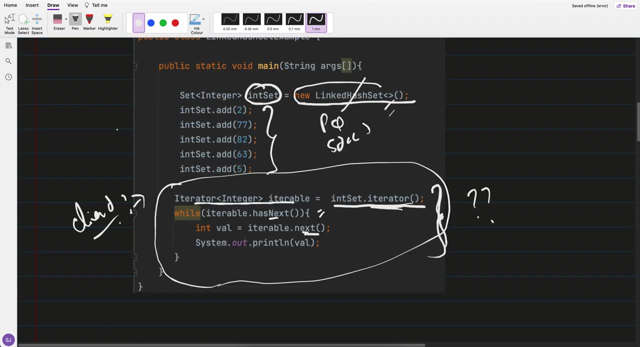 as many iterator are possible. ok, now, what is this aggregate? now let's see the third class which is present. so aggregate is also an interface. so aggregator is aggregate is something which collects the data. so here, in this example, these are the aggregators, and these are the aggregators and these are the iterators. so 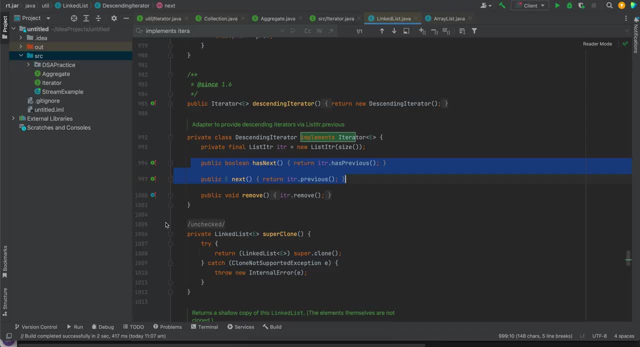 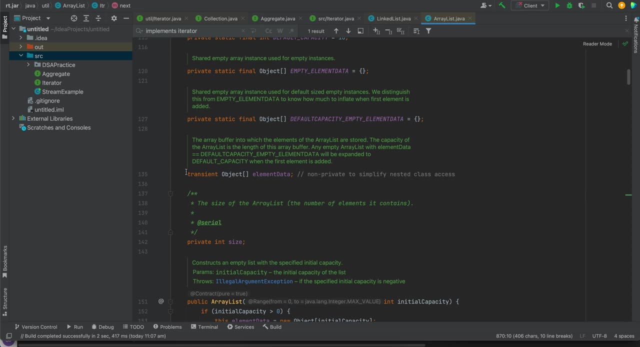 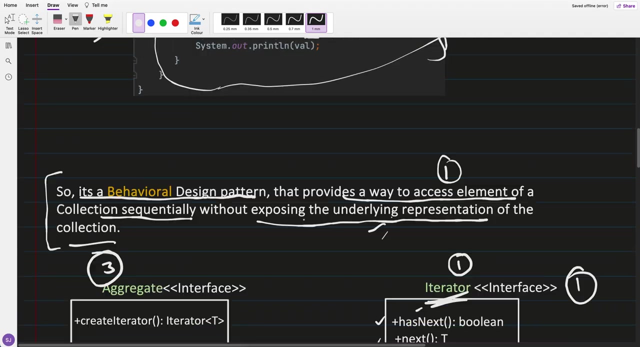 these are the iterators and these are the iterators and these are the iterators and these are all aggregate. priority queue, array dq. these are all aggregate, the array list. if you see that they are maintaining the collection, they are. this is the maintaining. they are maintaining a collection of the data. so aggregate is what aggregate is maintaining the collection. 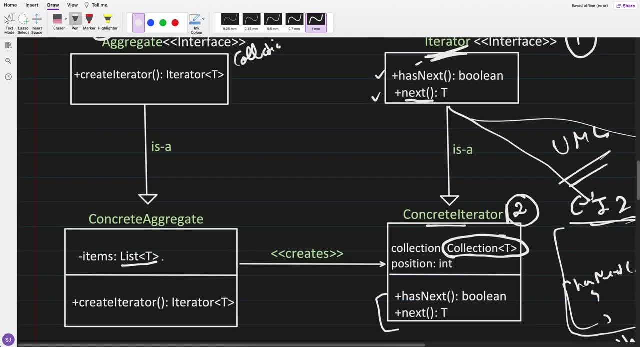 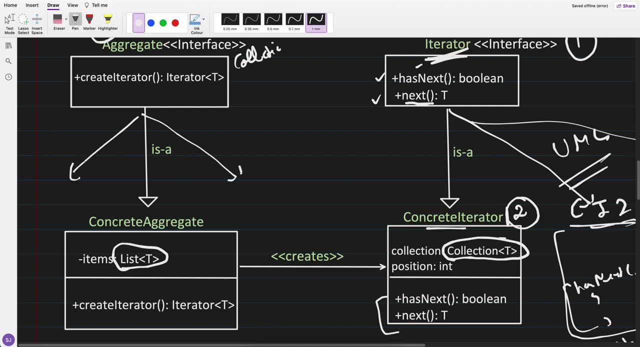 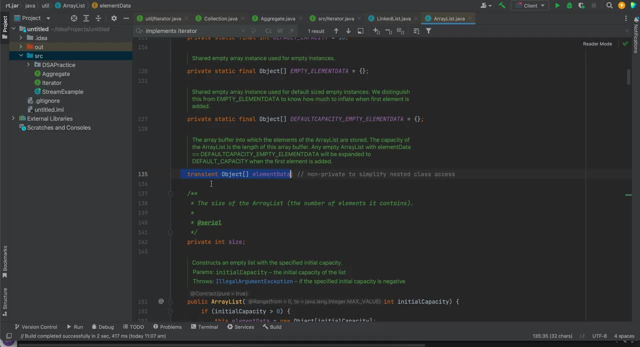 it is maintaining the collection here, the list, right. so this is just a one example. i have taken concrete. there can be many concrete. let's say, for example, if you are maintaining, let's say, array list, the, as soon as we have seen this, it is maintaining an internally using an array data structures to hold the data. 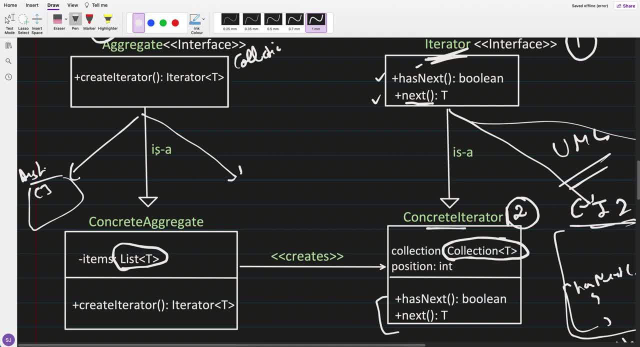 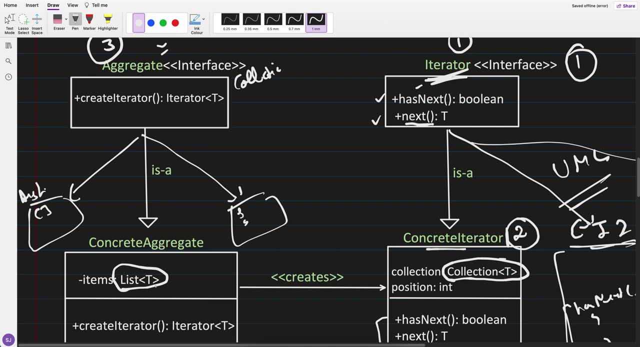 right, so it would be using array. maybe, if you are using linked list, it is using linked list data structure. so first node, second node, like last node, it is using that one. okay, but what does aggregate means is it is a collection of data. so for this example, i have taken it as a list. 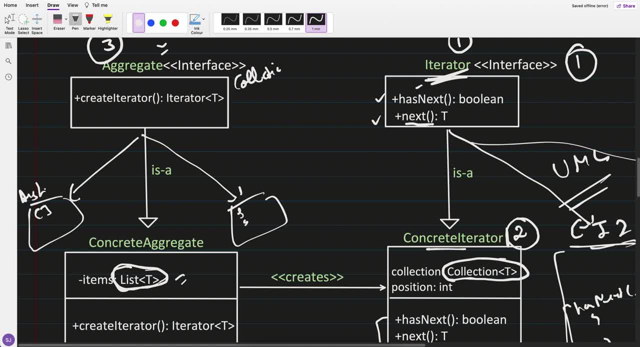 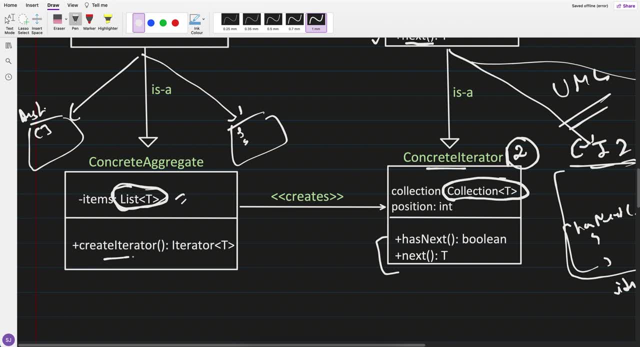 so i am using, as it is maintaining a list, okay, and this aggregate also expose the method. create iterator means it also provide a method which help us to iterate over this collection, right? so each, whatever the concrete aggregate you will write, they have to provide the implement data structure, right? so this aggregate means is it is a collection of data. so, for this example, 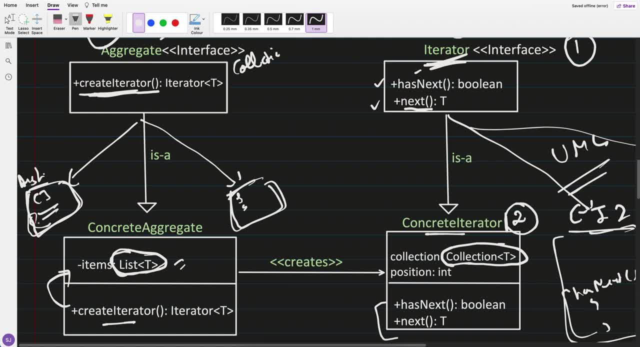 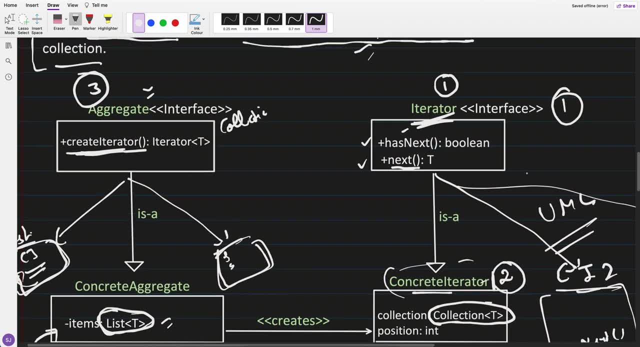 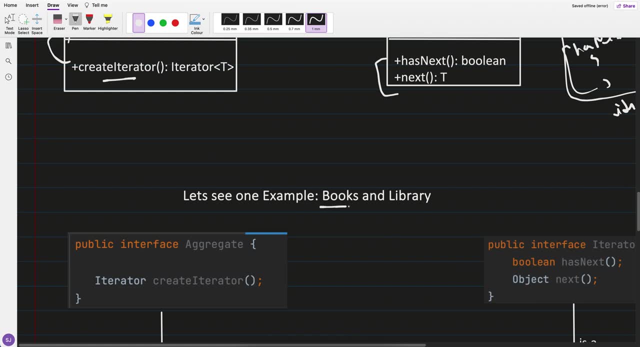 and they should return an object of this, which concrete iterator you should use to iterate that collection. now let's see an example. it will clarify fully, right. so now i am taking an example of book and library. so here i have created a book, very simple class like, which has a book name and 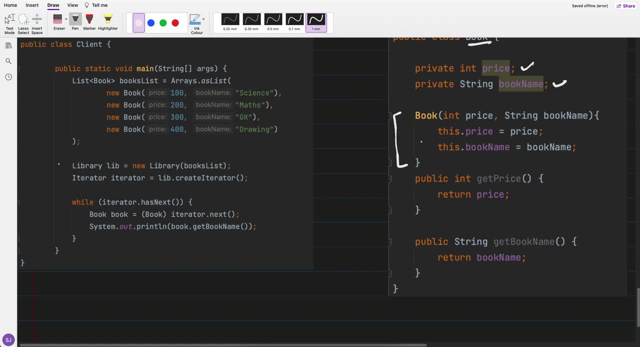 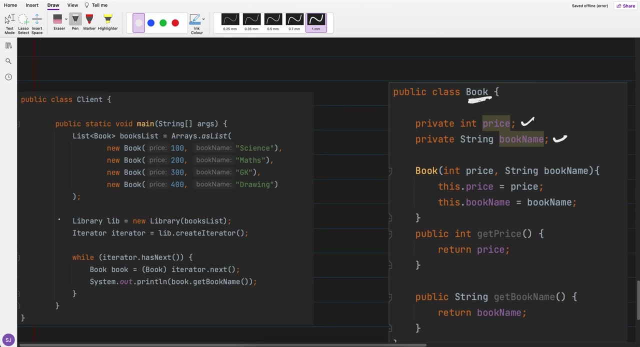 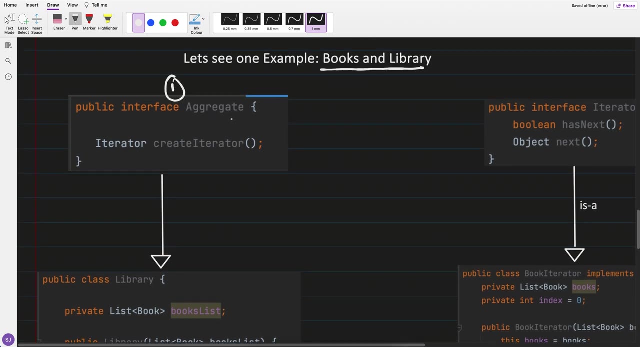 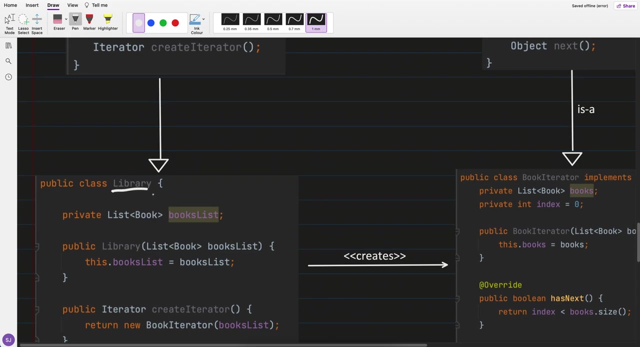 the price. the book constructor is used to set the book and price, and this is the getter setter, getter method setter. I am using the constructor. okay, so now here I am first creating an aggregate, right so aggregate. I have created, and its concrete implementation I have created is library, right so library. it is very similar to consider this as this: 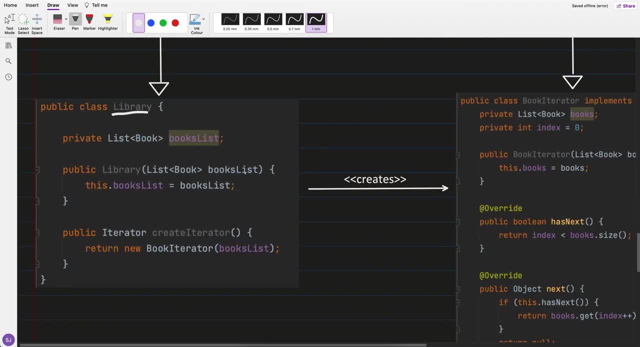 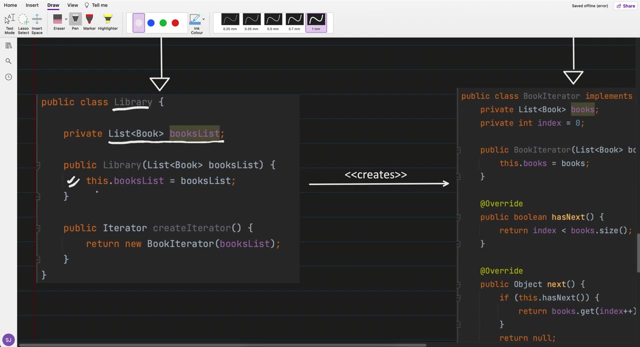 priority queue: Eric DQ. so they are maintaining a collection. so, for now, simplicity: I am using a list as a collection, so it's maintaining a list of what books. right, all these books. it is maintaining a list. so I am maintaining the list of books and using the constructor. 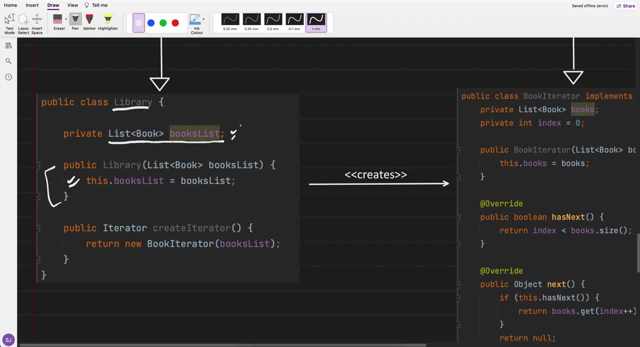 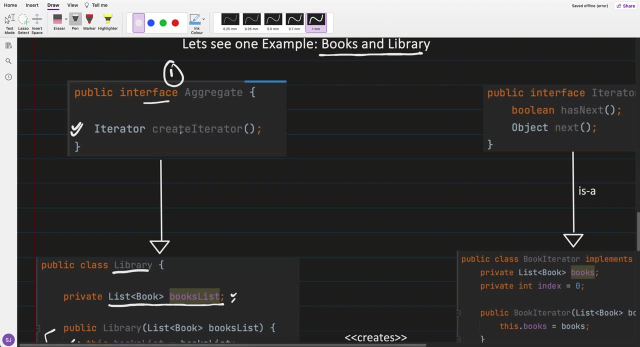 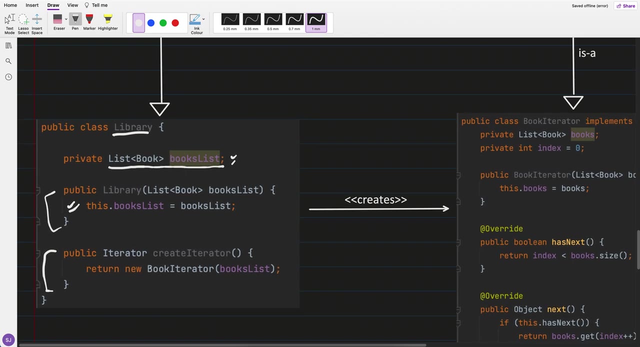 to set this variable. okay, and in the aggregate interface I have this abstract method where it is a created iterator. so a library has to implement, provide the implementation for this. There it has to tell, hey, which iterator you should use to access this. now, I told you right. 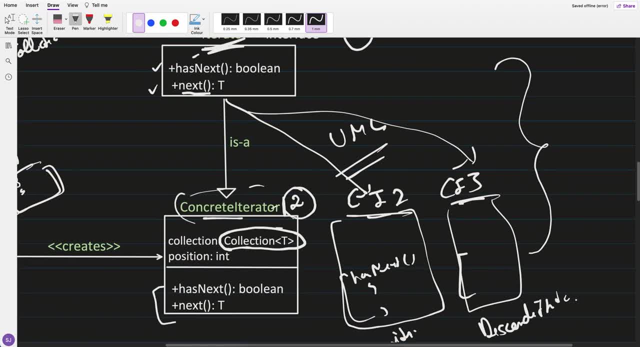 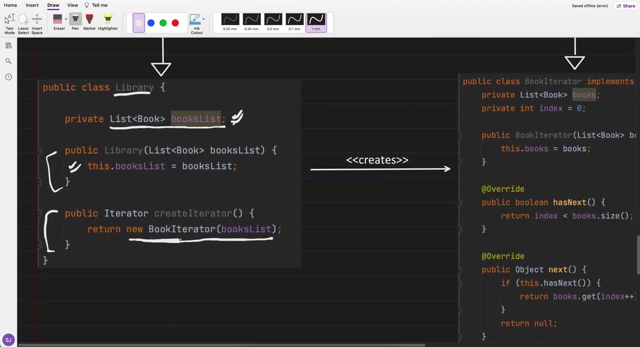 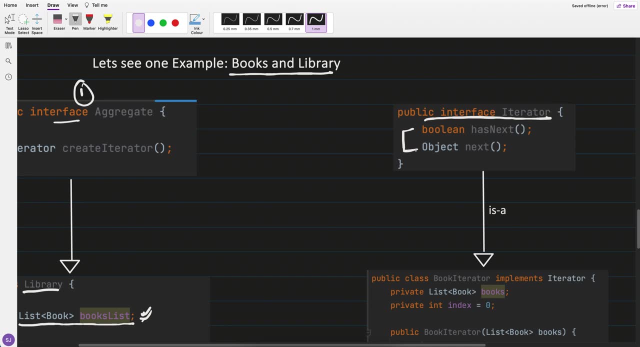 there can be so many iterators, right? so each aggregator has to choose its own iterator, depending upon what data structures. right, so I define the book iterator. so here now we see that in an particular interface iterator- these are the two methods- has next and next. so I have written book iterator which implements this iterator. 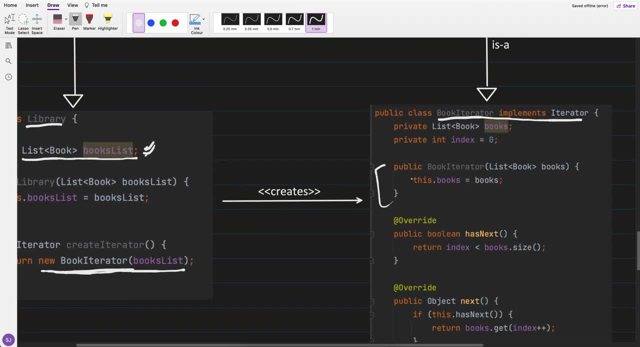 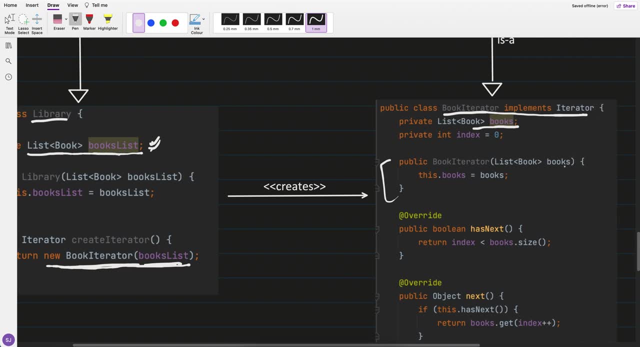 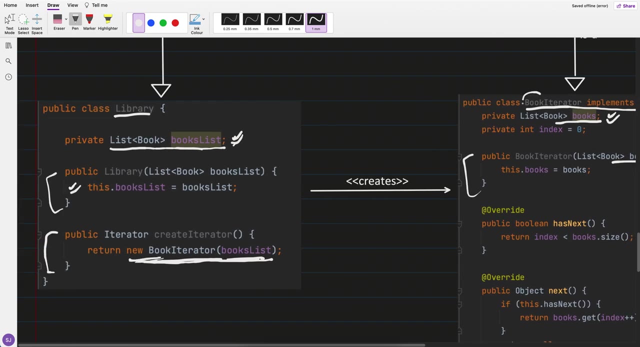 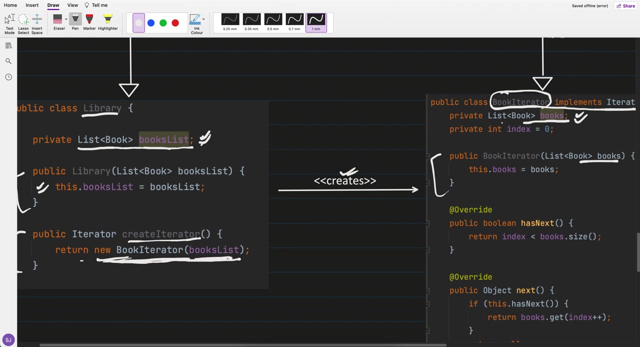 Right and it has the collection which it has to work on right. so I pass this book list from library in this constructor and this gets set right and it will return this book iterator object. it will return this so it creates. so this create iterator will create the book iterator for this and return. 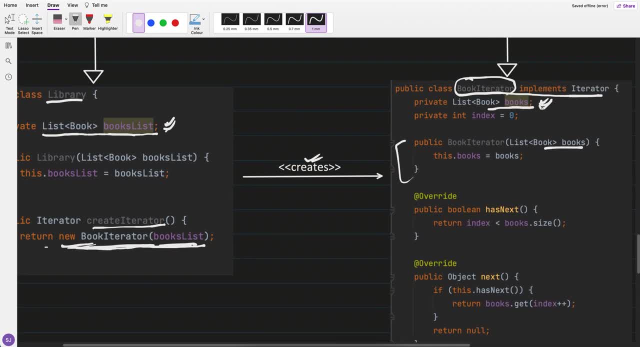 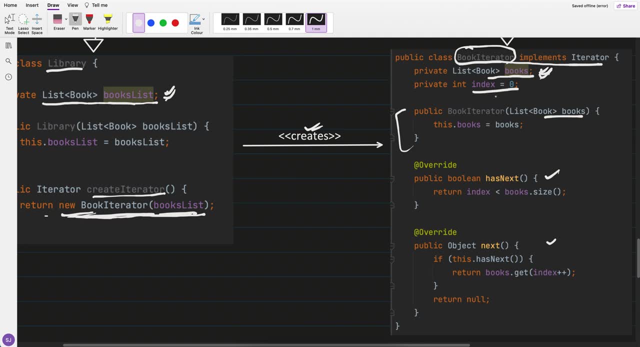 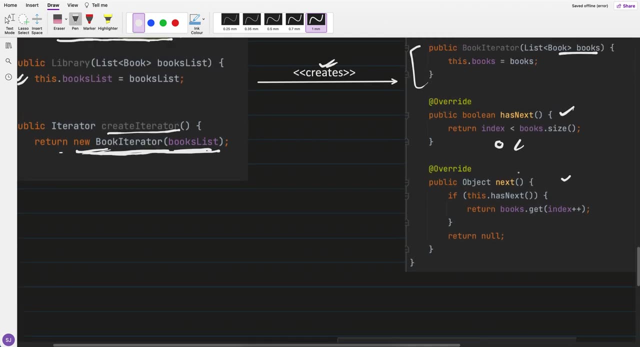 Now using this object. We can access over this list of books using has next and next, so has next. you can say that. okay, currently I have put index equals to zero, so has next is zero is less than book size. let's say they are. what is the book size? so, for example, one, two, three, four. yes, there. 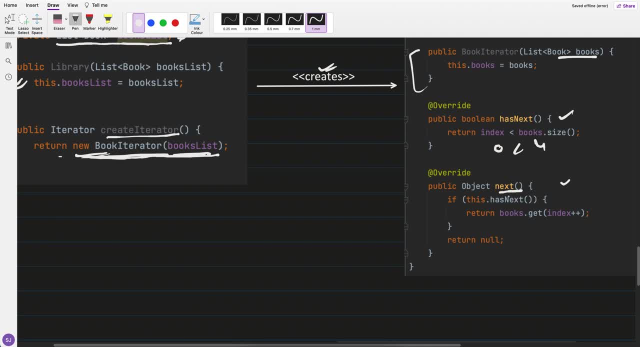 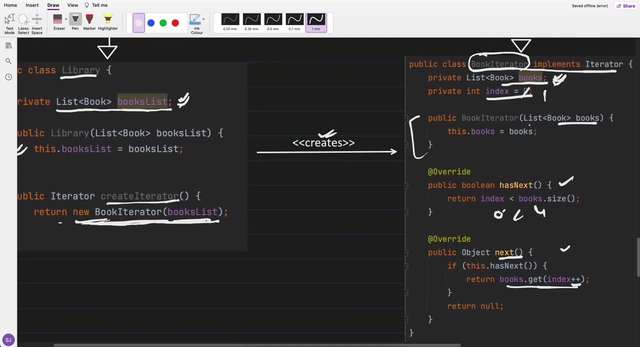 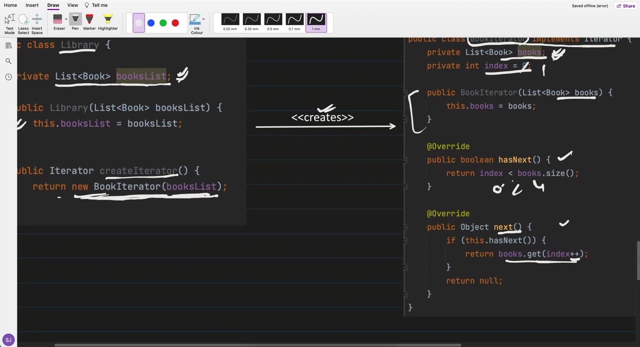 are more books. so whenever somebody do next, I will get that book and increment the index. so index will increment, so it will become one. Then somebody do: Is there any more Data? yes, it is more data is present, so it will return true. then somebody do next it will. 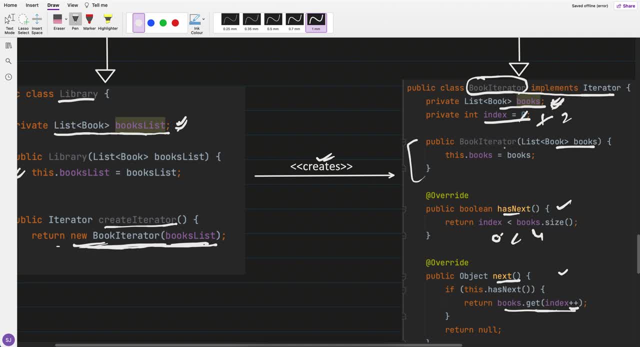 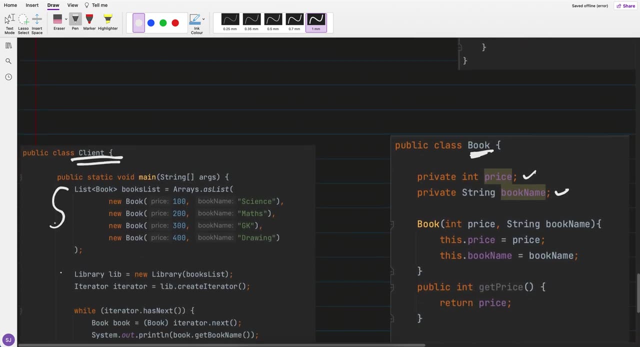 fetch that and increment it. it will go to like this: so this book iterator, if you see, help us in iterating the list of books, this collection. So this is the client. so in the client, I have created a list of books. I have created a list of books. 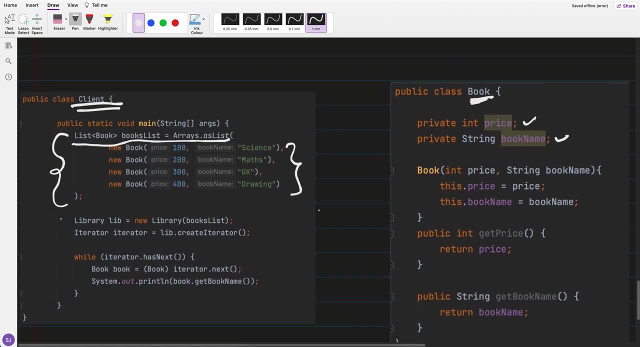 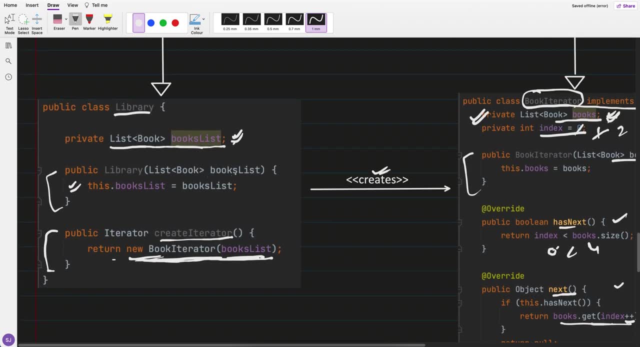 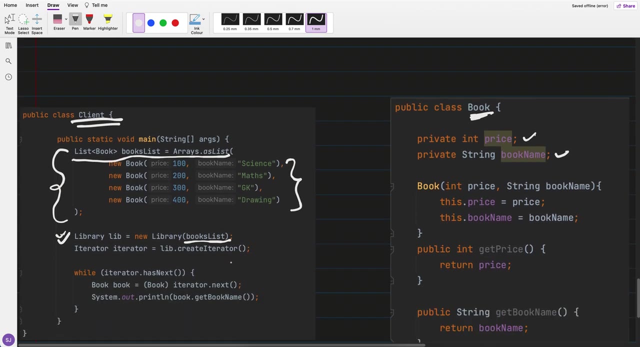 Right, I have created a library and in the library I have said this books, okay, so now my library is set. I have said the books like this library has these other books list. Now, if I want to iterate now, this is the client right? so client doesn't bother whether what. 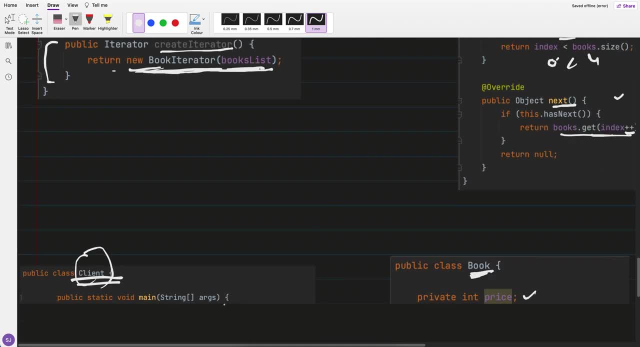 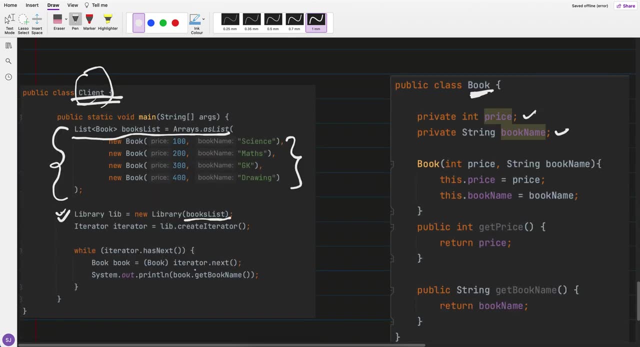 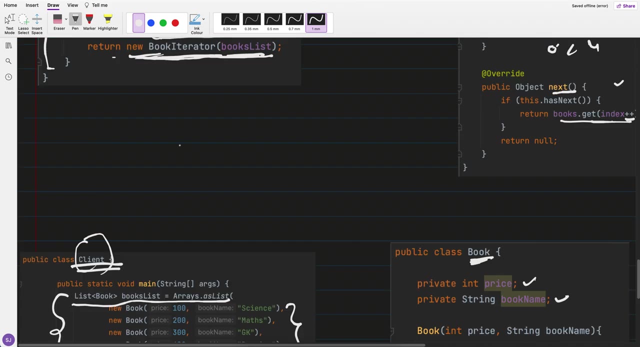 internally. how this library is storing this list of books, I don't care, I want to iterate it So it can invoke the create iterator method, right? so I call the create iterator method of the library. I got the iterator object, so what object it return? new book iterator- this. 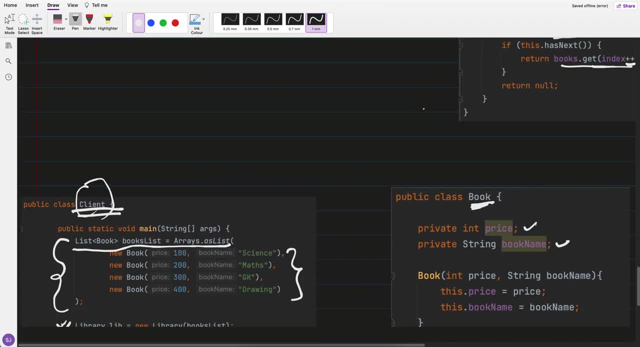 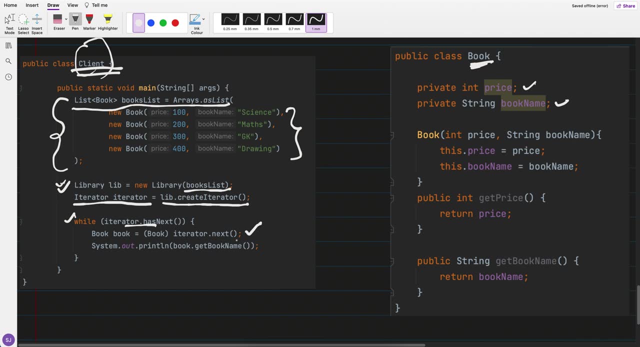 one right now. what I will do is I will do: hey, has next, yes, if there is more value, dot next, return me the value and I will print it. then again, loop will go: has there more value? So I will say yes, then it will get the value dot next and then print it right and using. 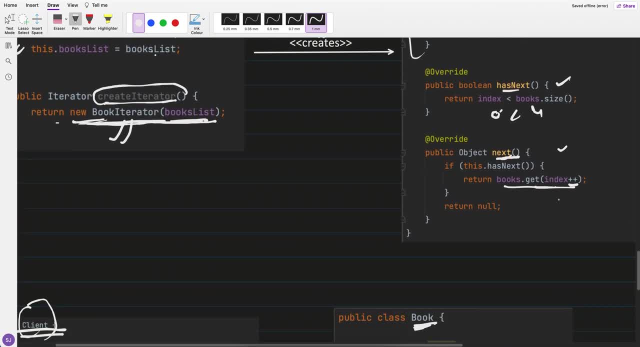 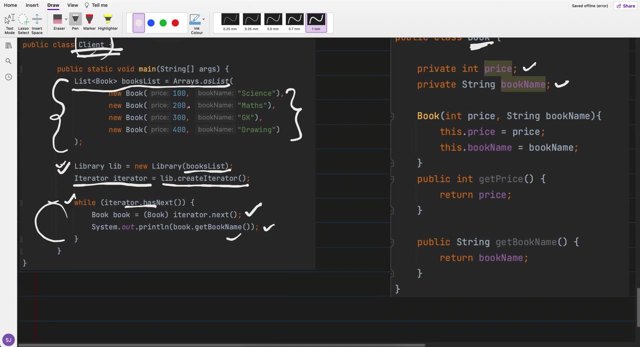 this index. every time I do, next index will increment, so I will get different, different value and once the index will be your four means we are iterated. all the elements it will come out of the loop. Now there is doesn't matter. so currently, today we have only library. now let's say you have 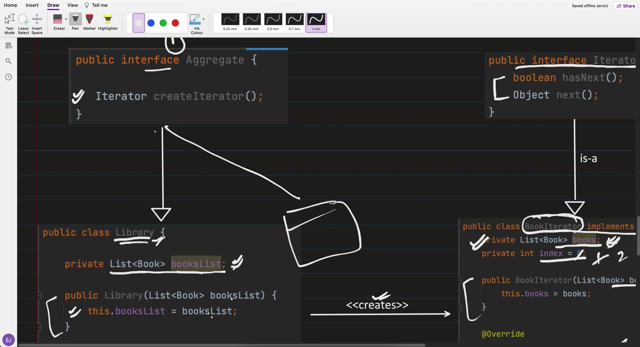 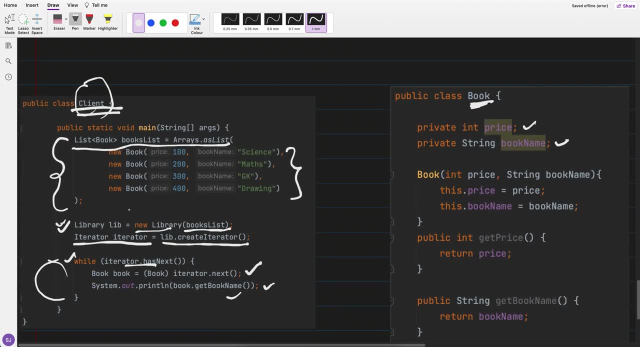 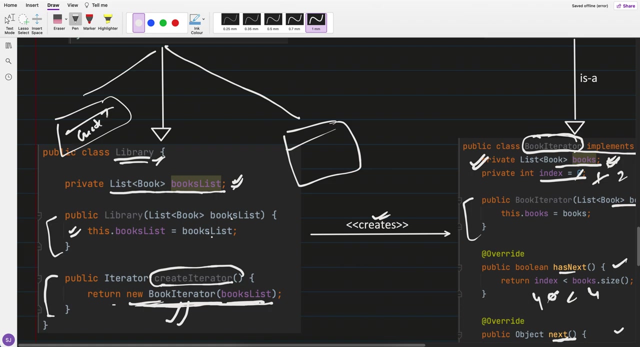 some other aggregate- concrete aggregator or some other concrete aggregator right. So now doesn't matter. today you have created new library. tomorrow you can create some new, some other class, concrete aggregator, two class, some other class. this would remain the same. why? because they would be. they would also have to implement the create iterator method. 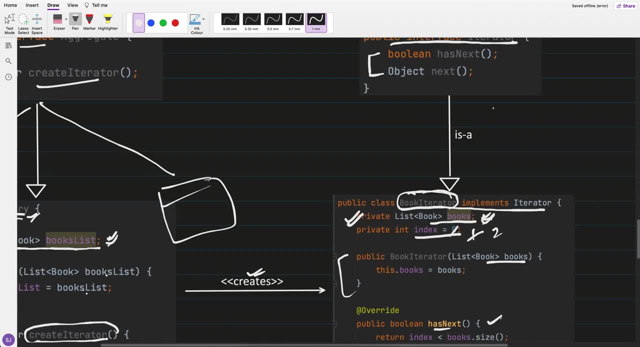 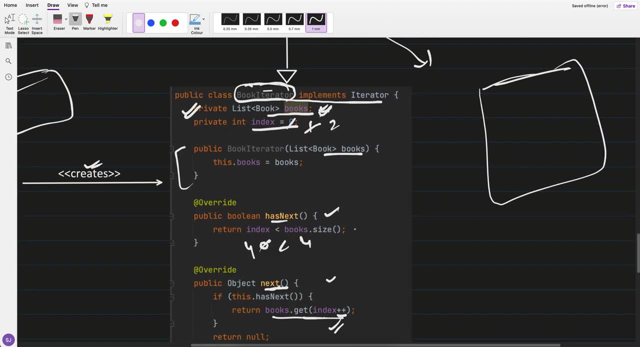 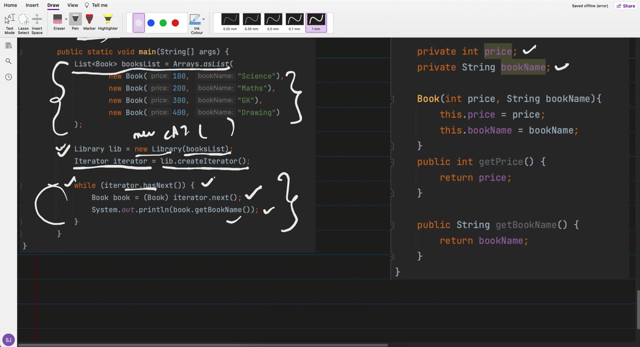 this and they should provide which iterator to use. Okay, Either book iterator you want me to use or some other iterator you want me to use, and whichever iterator will do that has to implement this two methods. has next and next. right, So for this client has next and next. only it has to know what they will do. has next. 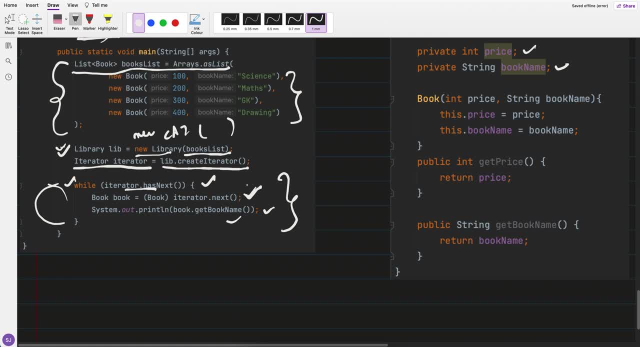 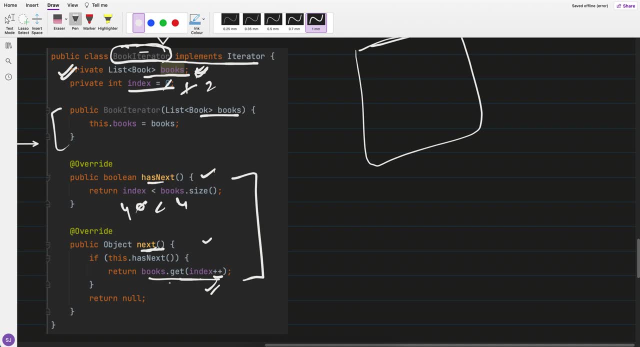 if true, it will return. true. if there are more value next, will return me the value. but it doesn't have to understand what is the logic I have to do to fetch the next value. is it an array or linked list or data structure like, whatever? it is a stack trees, whatever? 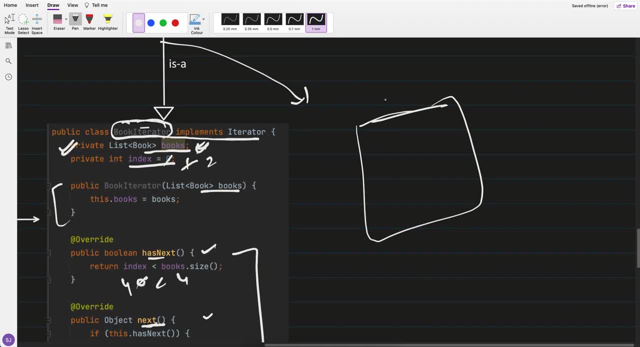 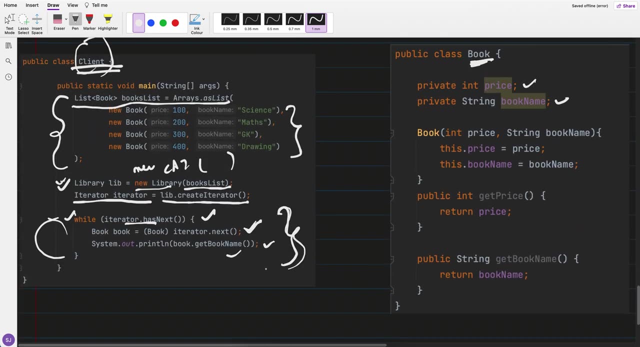 there I have stored the data. all this logic would be present into this iterator, concrete iterator, to has. next it will do, and next there that there will, it will have the logic to fetch right. So for client, this logic will remain the same. you got it, so now let's see the collections. 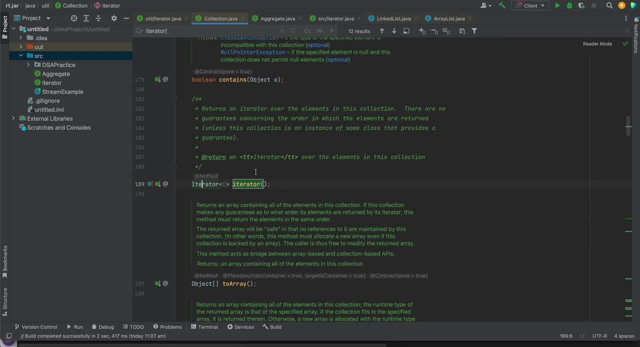 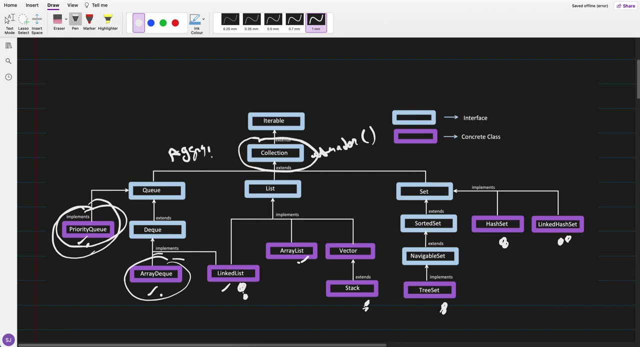 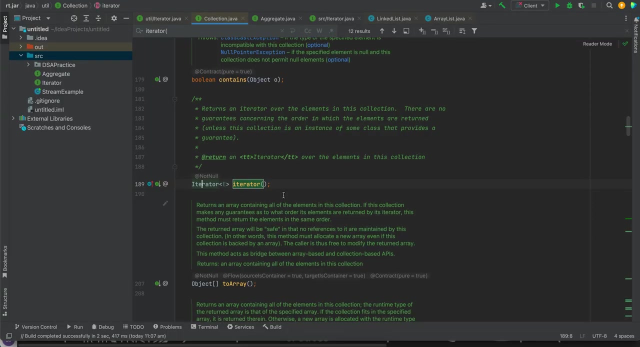 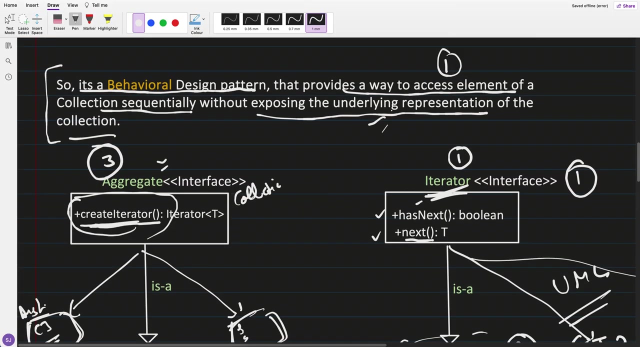 here also. So Here the collection, this is your word, this is your aggregate, right aggregate: expose the method, create iterator. so there it has: expose the matter, iterator, right. so we have given the name: create iterator. it has given iterator. now there are concrete aggregate. so what are the concrete aggregate in this collection? these are the concrete classes. 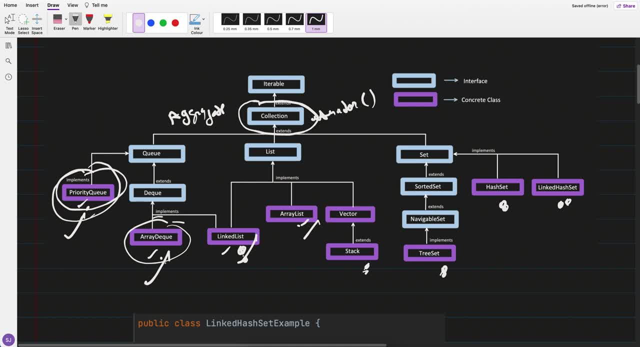 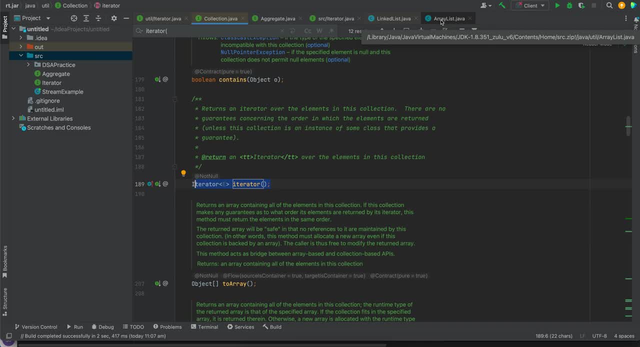 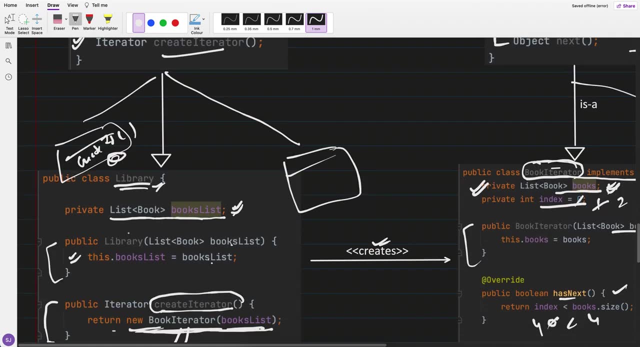 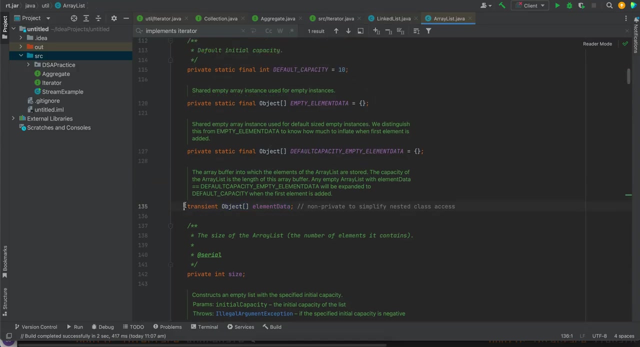 this all, pink, purple, one. So these are all the concrete aggregator. so now let's go to any, let's say ArrayList, right, so here, concrete aggregator, what it has, it maintains the collection. it maintains the collection. so I have already showed you that. say: this is the ArrayList. it is maintaining. 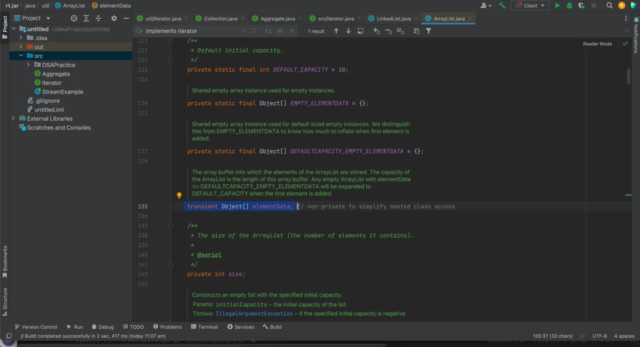 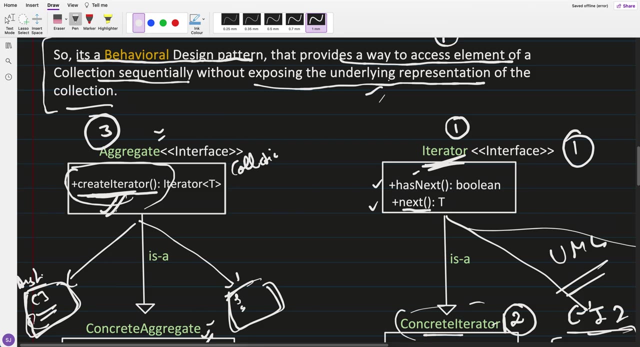 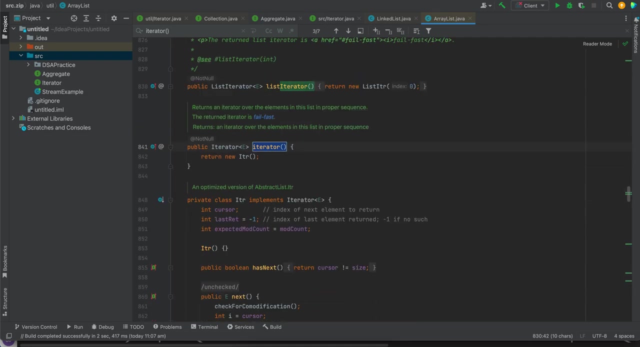 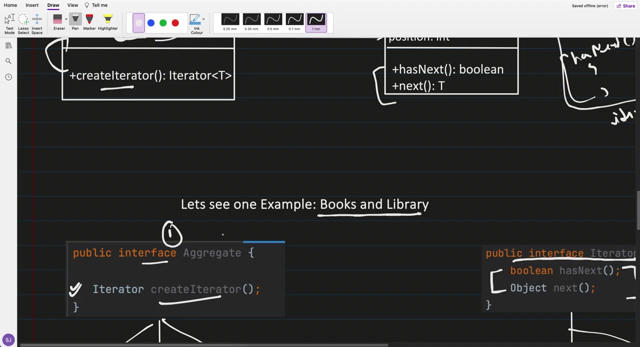 the collection. so it is: keep on storing the data. Now, Now, Now The aggregate, concrete aggregate, also has to implement this. create iterator. so in this example, it for the grave, so iterator, it has to implement. okay, so here, if you see that it has implemented the integrator, so it is returning the new iterator object, so like: 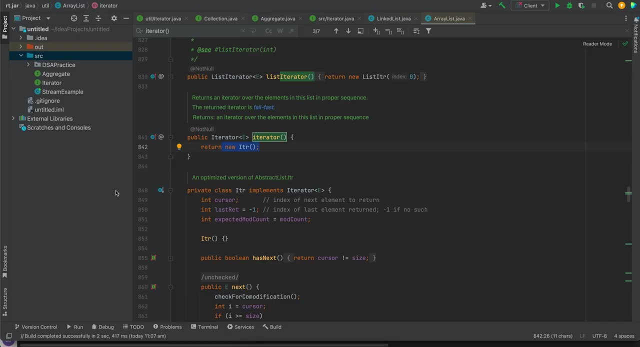 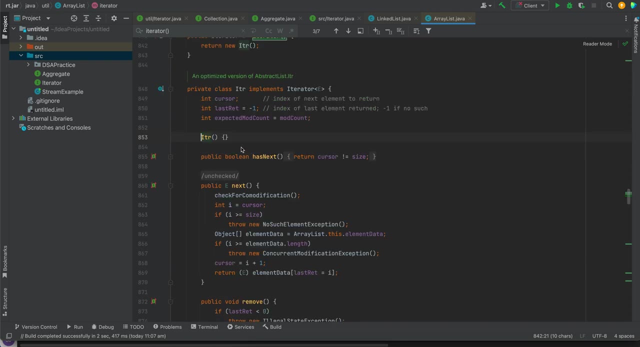 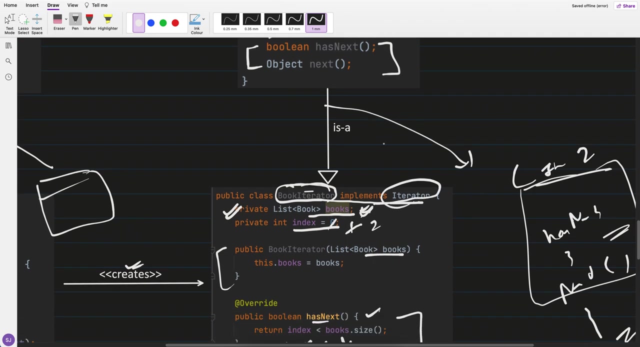 we are returning the new iterator, right, it is returning this new footer, но to iterate the collection. so now let's go into this one. so here, it implements the iterator. so this is this part. so it implements this iterator. so iterator is an interface. I have already showed you which has has next. so ITR is the one. 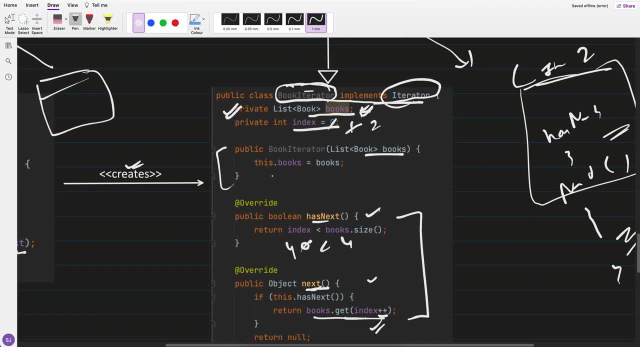 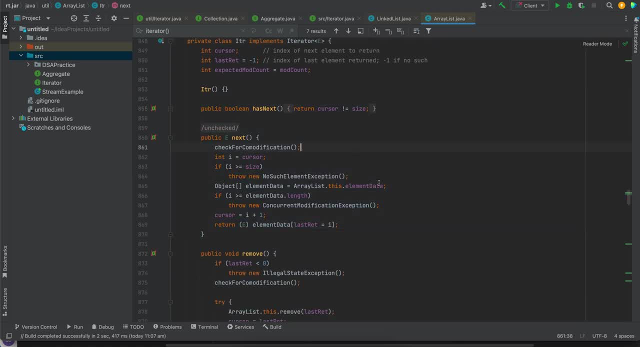 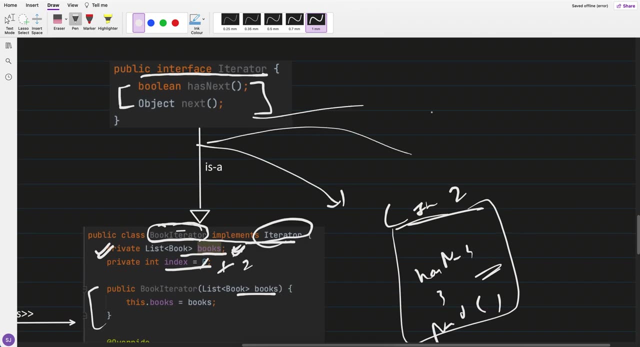 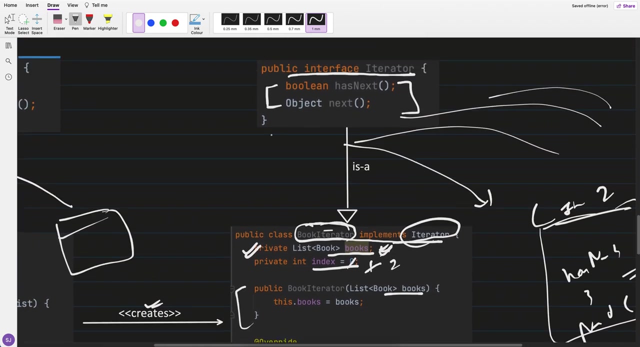 which implements this and it has has next and next, like how to access it. it is defined so it is working on this elements data right. so if there are more iterators, you can add it right, and if there are more aggregate, you can add it. for each aggregate, you can define which iterator to use and with this, client can. 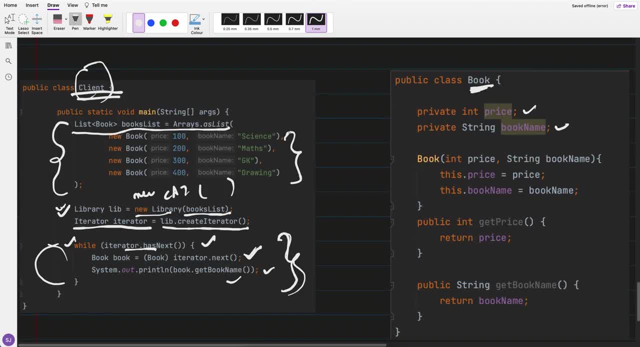 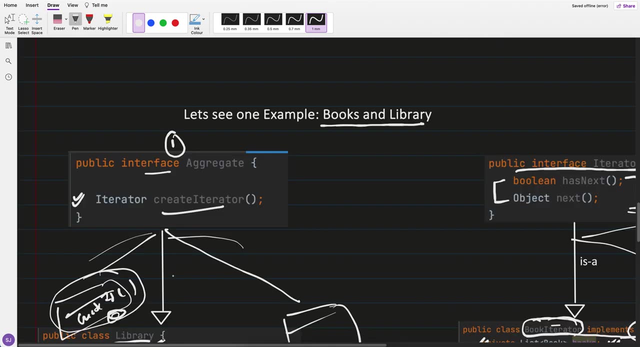 access without worrying about what data structure is used internally to store this data. it doesn't have to bother it- with the help of iterator- that is what it is working on right now. so now, if you do of the iterator pattern, it can simply access it using this. okay, i hope you got it. it's a very like. 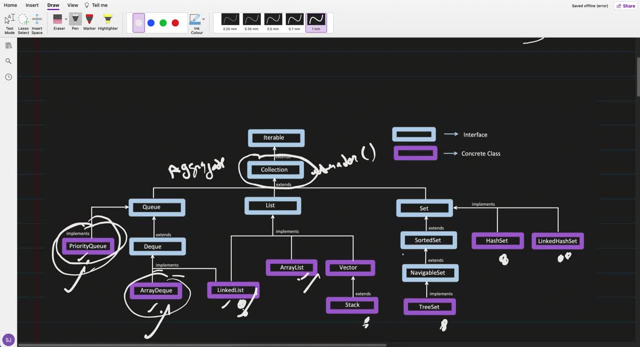 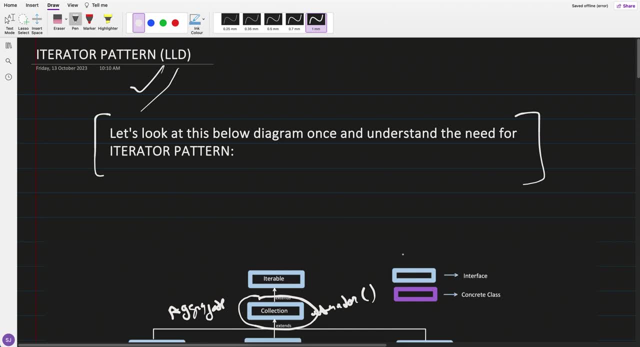 the biggest client of iterator pattern, you can say, is the java collection itself. so do practice it once more time and you will find it very easy. so it's very, very straightforward and if there is any doubt, uh please ping me on uh comment section. we can discuss more. thank you guys. bye.